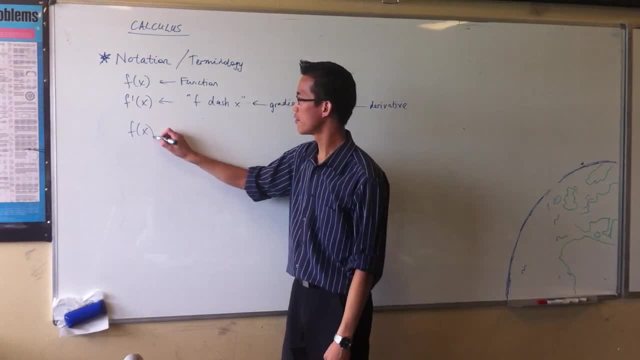 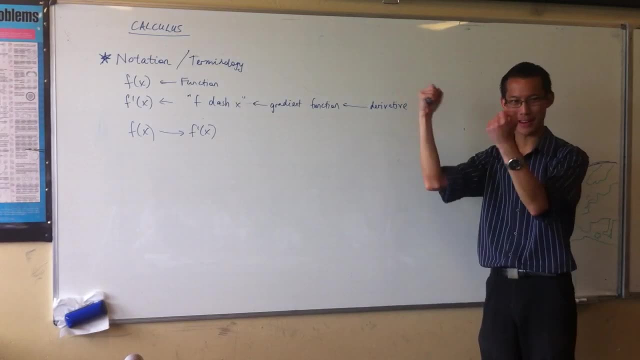 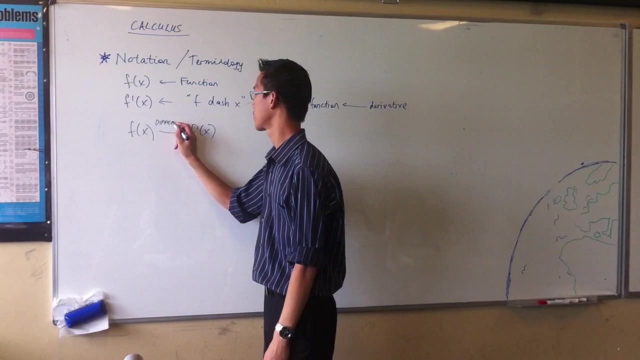 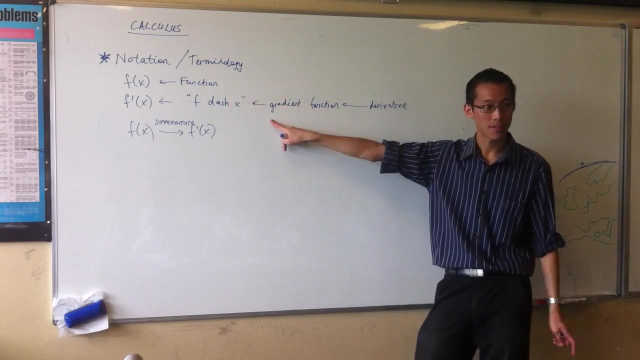 The process of going from f to its derivative. okay, This process is not called deriving Stupid mathematicians and their use of English. It's called differentiating, Okay. So to go. So to go from a function to its gradient function, to go from f to f, dash, we call that differentiating, okay. 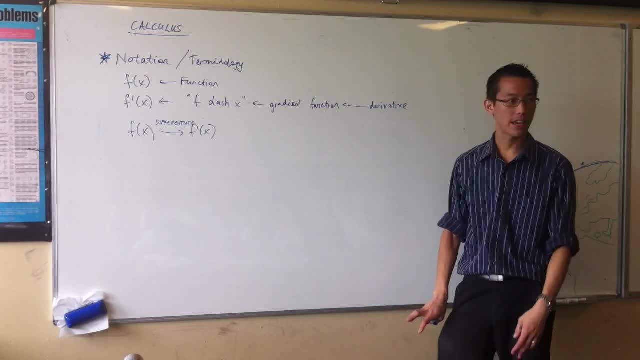 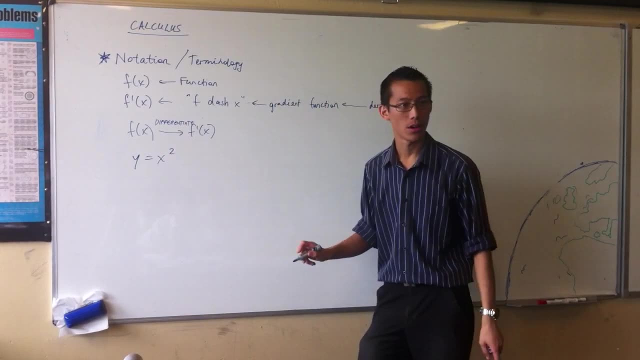 Now, all of this is in terms of f's, okay. Usually when you get a function, we say y is equal to something, right. Like say y equals x squared, okay, So this is again that's a function, right. 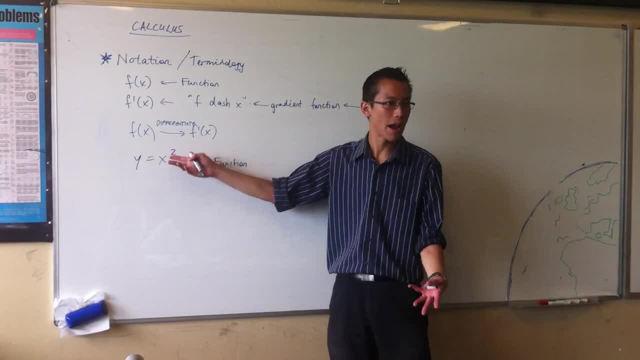 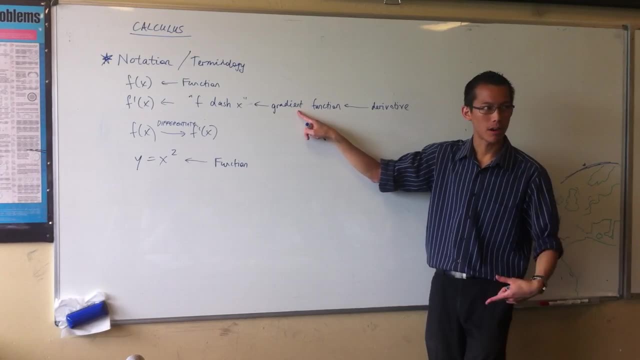 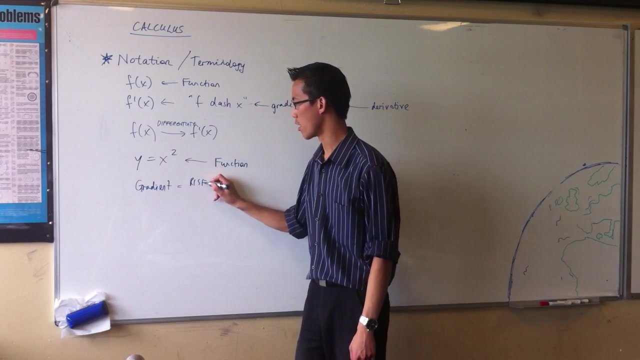 But when you want to talk about its gradient function, there's another way of describing it. There's no f's here, right? So what would I say? Gradient is all about rise over run, Rise over run, okay. So therefore, gradient right is rise over run. 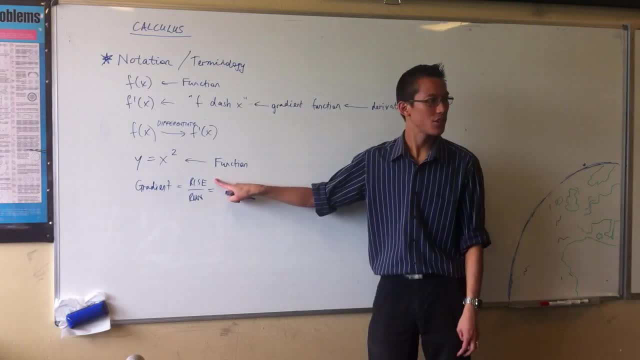 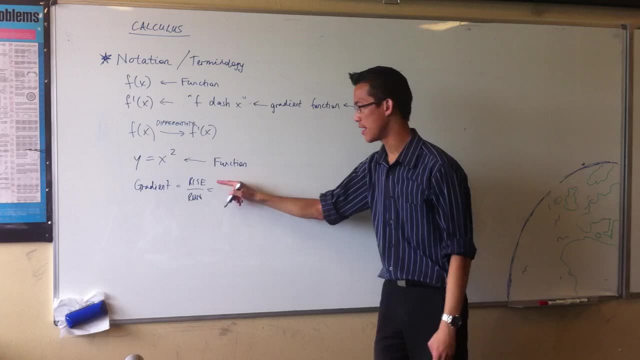 Look up at this one because this is important. okay, Rise is really just a way of saying: how is my vertical distance changing, How is my y value changing? right, So rise, instead of saying that, I could say the change in y. 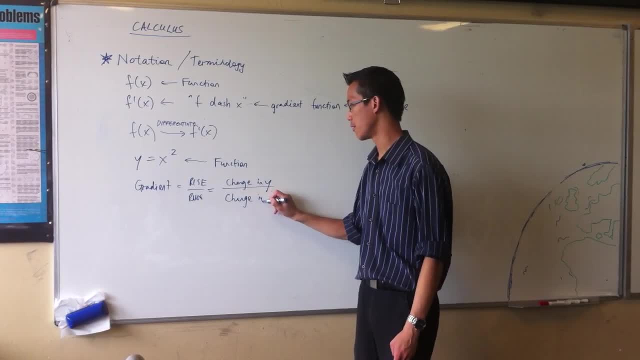 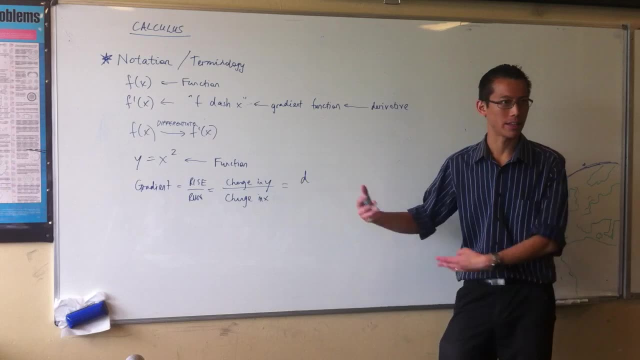 divided by the change in x. okay, But this is very long. So instead of saying change in, we say d. actually we mean delta, like Greek letter, and we see this in science as well: in like a chemical equation. 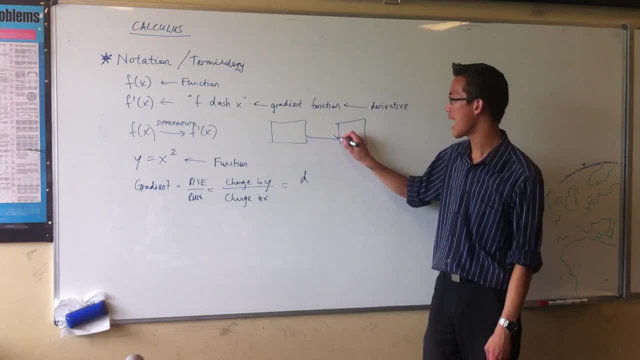 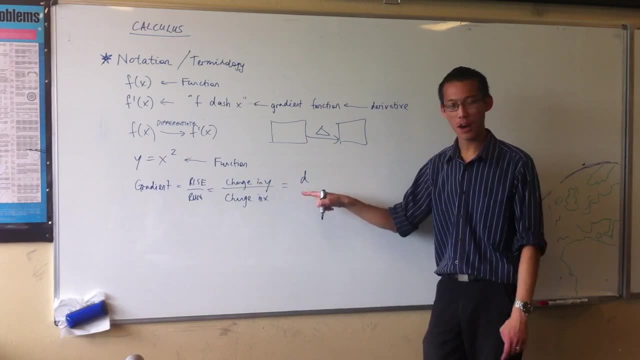 You've got some chemicals and then they turn into something else and there's a reaction, a change in the middle. right, That's just the capital D in Greek: delta. okay, So a change in y. we say we call that dy okay. 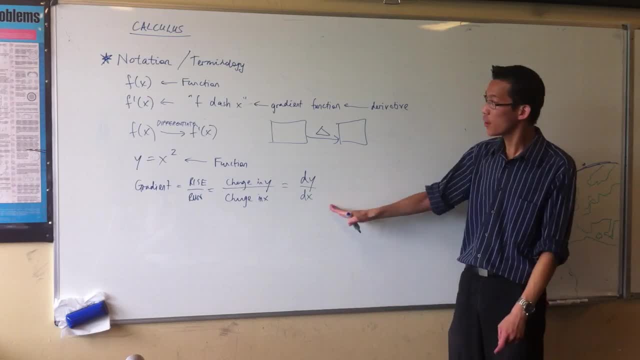 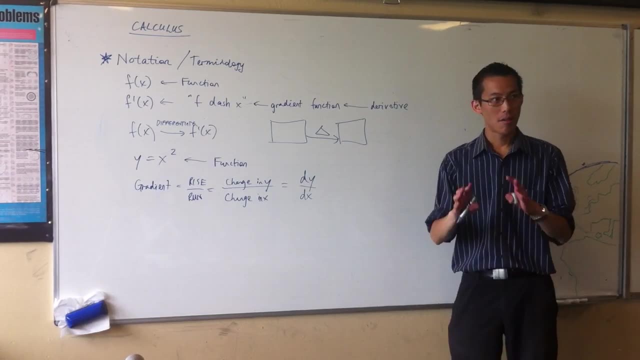 And the change in y is okay And the change in x we call dx, right? So this is another way of saying the gradient function or the derivative. okay, It's the same thing. okay, But let's make this a little more right. 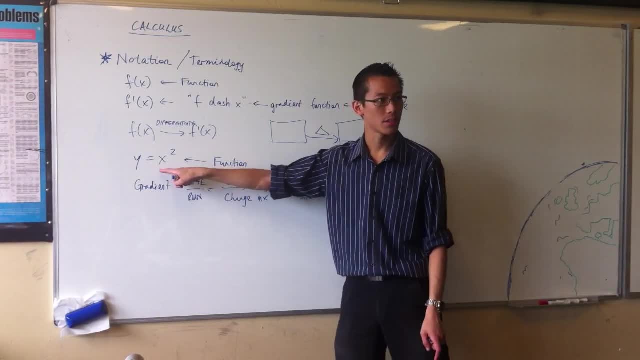 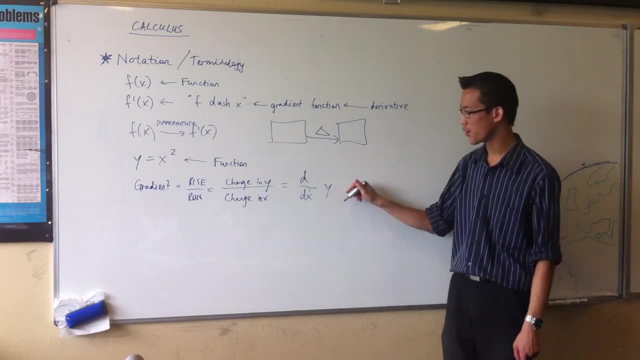 This y, right, it's actually equal to something in terms of x. okay, So I can write this as putting that y out over here. So y is the function I am differentiating, okay, And d on dx. 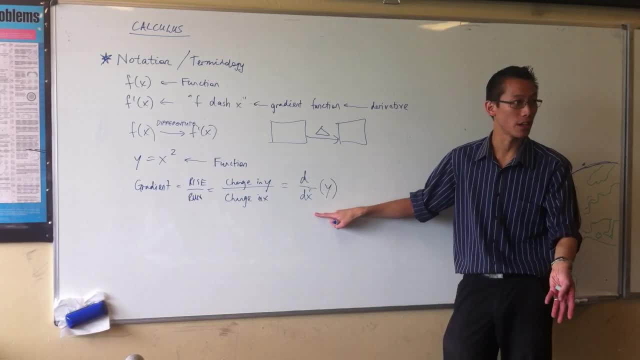 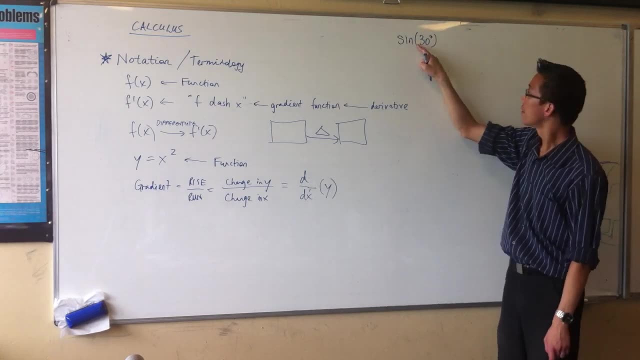 So d on dx is the process of getting the gradient function differentiated. okay. So it's a bit like you know, when you see sine of 30 degrees, okay, 30 degrees is the thing that you're doing an operation on and sine is the operation, okay. 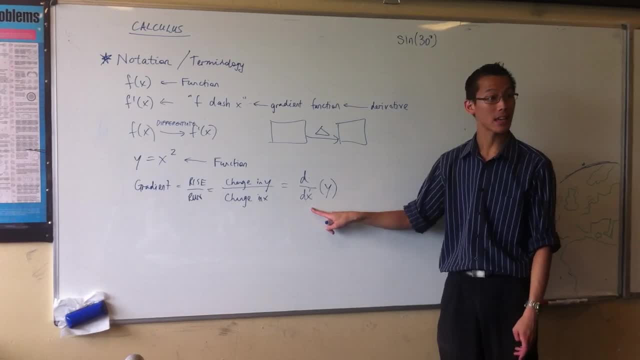 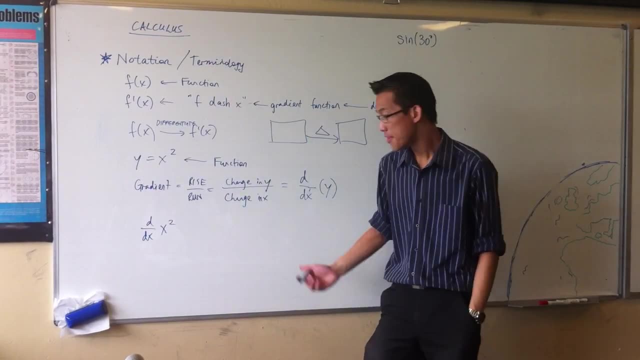 Well, if you want to differentiate y, you put a d on dx out the front, okay. So, for instance, I could write d on dx of x squared. That would mean differentiate y, right. So I could write d on dx of x squared. 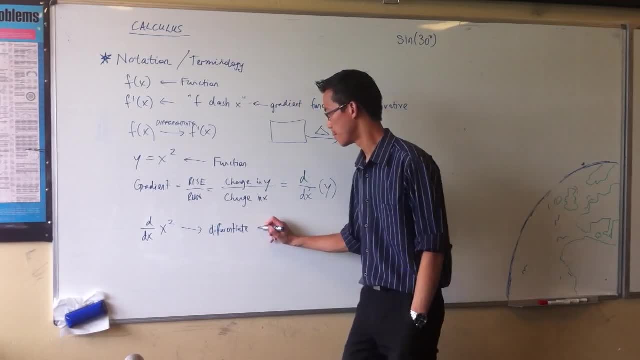 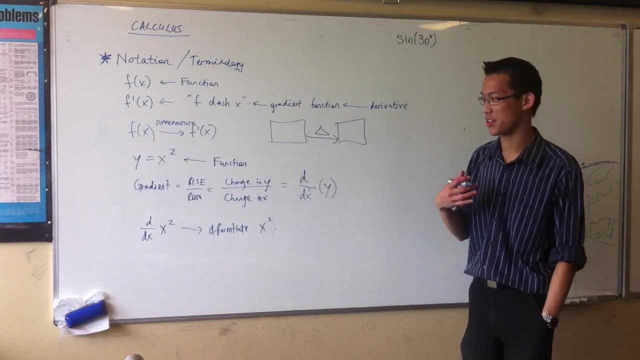 So, for instance, I could write d on dx of x squared. So I could write d on dx of x squared. Okay Now, this is a really crucial one, because lots of people make this mistake. I know I did back when I was in year 11.. 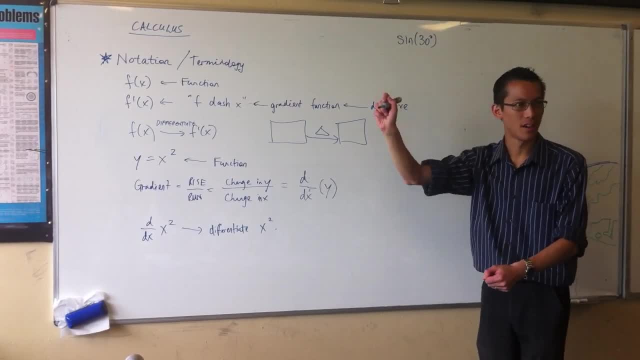 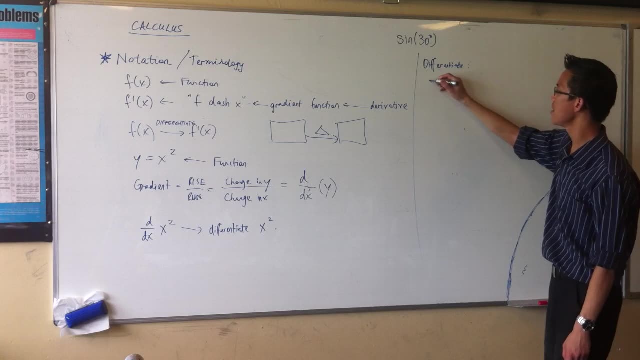 When you're trying to work out the derivative of something and you're just writing down your answer. okay, The question says: you know, differentiate or find the gradient function, and then you've got a whole bunch of examples, right? 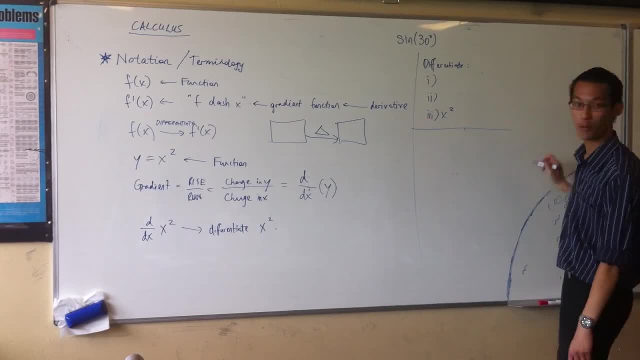 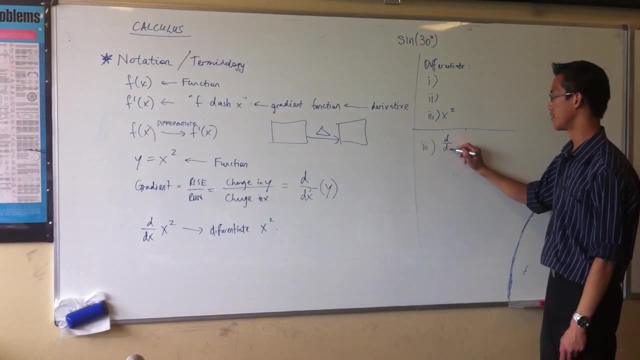 Okay and say the third one is x squared okay. So you get down to writing your answer And you say: well, the way to write a derivative is this right? So you write d on dx, right? It's better than saying dy on dx because there is no y right. 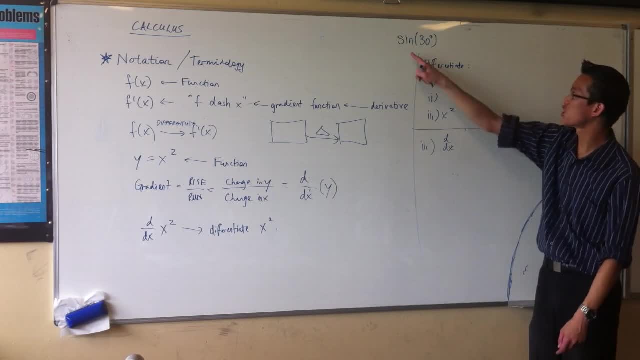 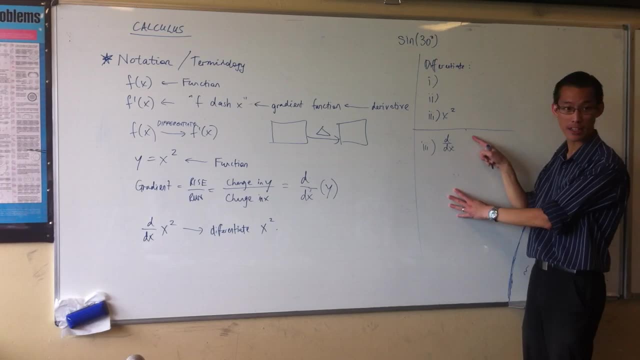 But it also doesn't make sense on its own. It would be like saying sine on its own, Sine of what It's an operator, It has to do something to something. There has to be an object here, right? So you'd have to really say d on dx of your function. 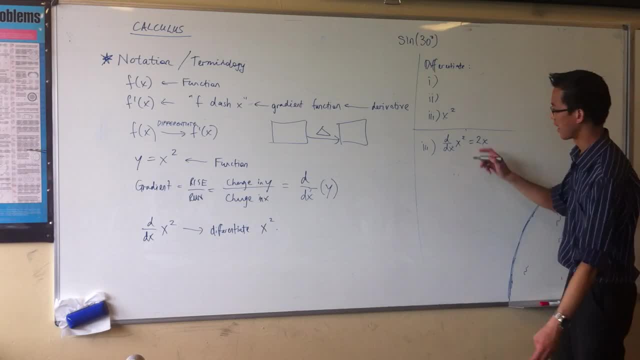 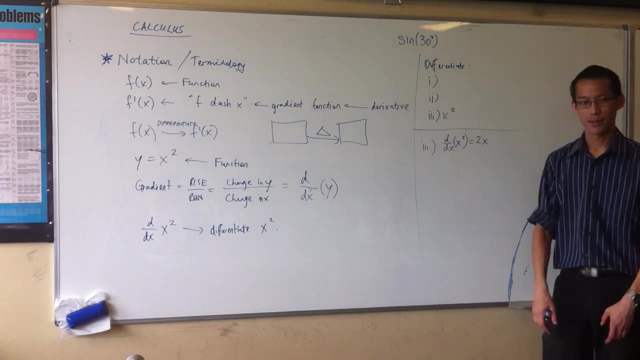 It's 2x, Right, it's around the x squared. Okay, Strictly speaking, when you've just got the one term, you don't, but we put them in to clarify, okay. So, um, hmm, One more thing I want to put down. 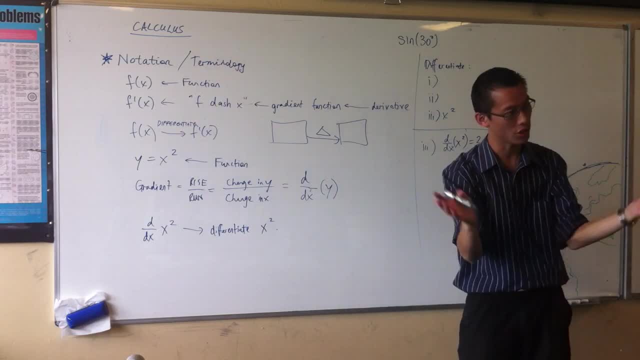 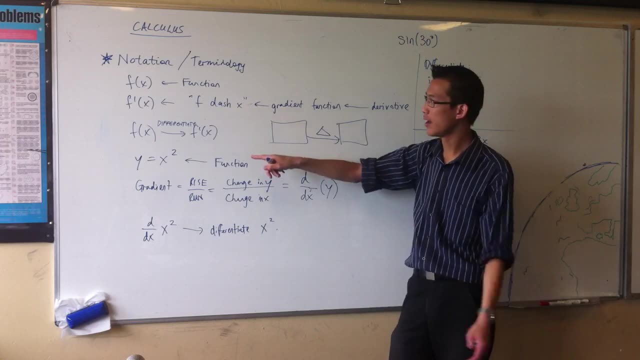 When you're finding the gradient function. often they don't want the function. they actually want the gradient at a particular point, okay. So, for instance, if I want the gradient at x equals 0,, okay. Instead of saying f dash x, they'll say: 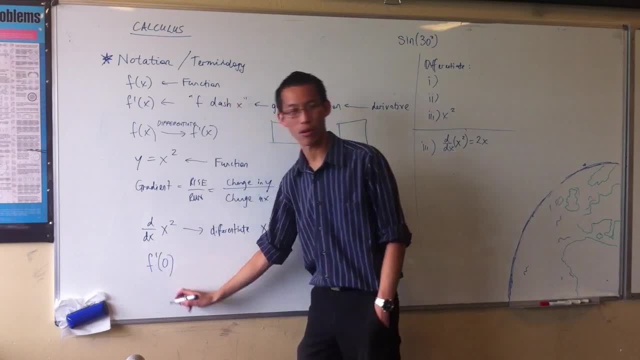 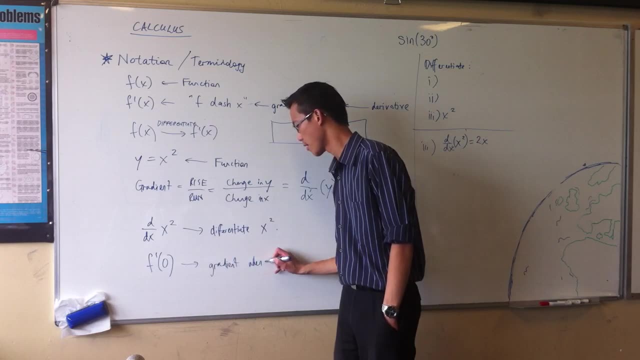 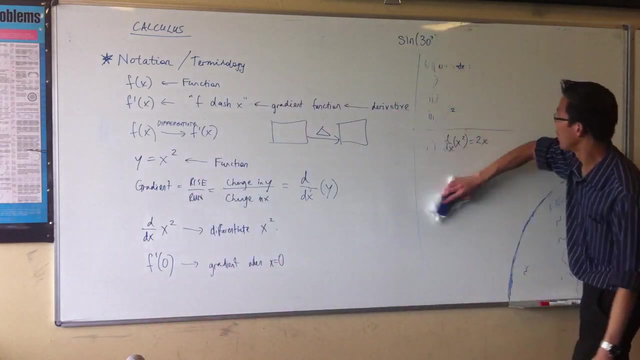 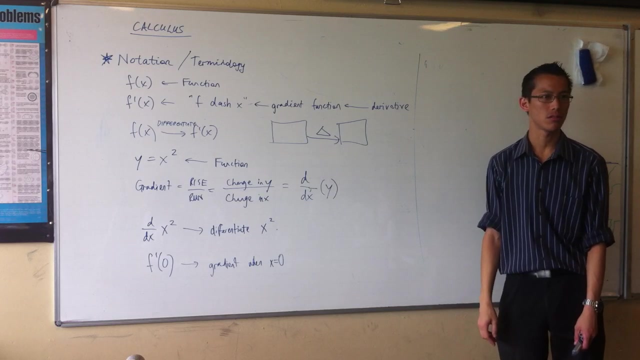 Okay, Um, f dash 0,. okay, That means what's the gradient when x is 0?? Okay, So all these different ways to write things. okay, You want to be watchful for them. Um, and even though we've all been talking in terms of y's and x's, in a sense it doesn't really matter what letters you use, right. 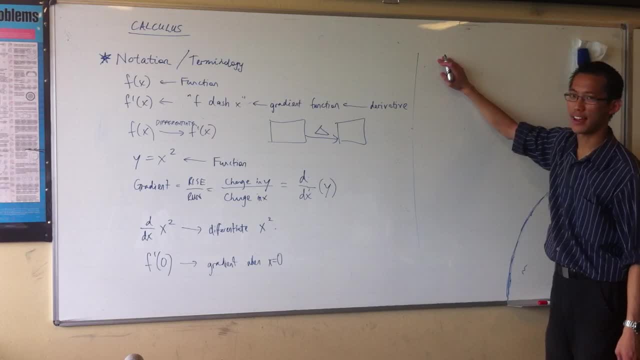 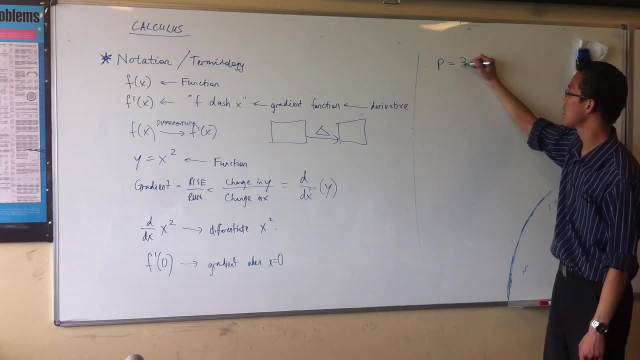 So, for instance, you could have, like a, you know a, let's see, Hmm, Um, a position function in terms of, say, your velocity, Position velocity. Okay, I can still find the gradient function of this. 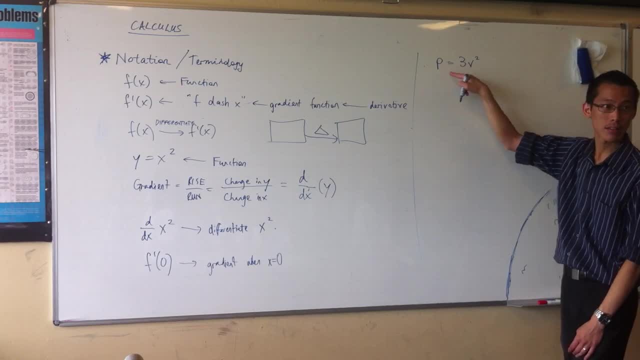 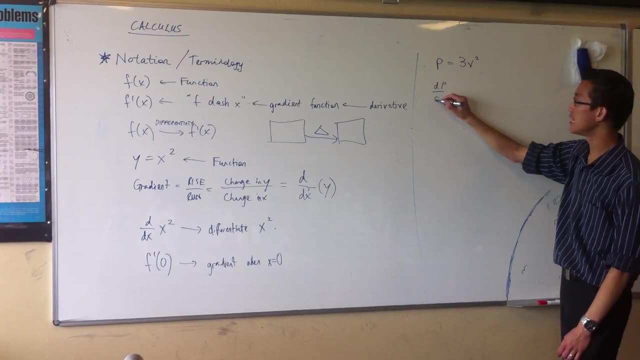 I can still differentiate, but it won't be dy and dx. Okay, It won't be dy and dx, It'll be dp. that's the thing out the front, right On d. well, what's the other variable, dv? 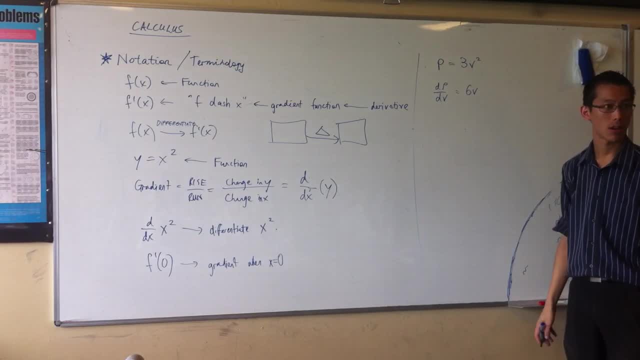 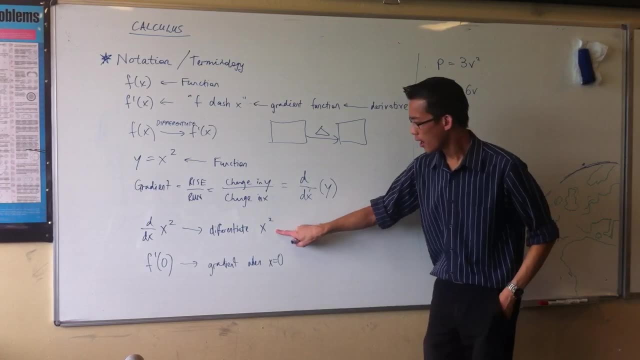 Okay, And that'll be 6v, Okay, Okay. So what we're doing here versus what we're doing here? um, let's see here, Where did I put it? You're differentiating x squared here with respect to x. 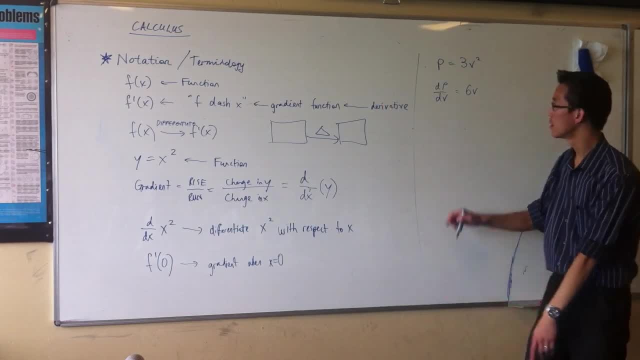 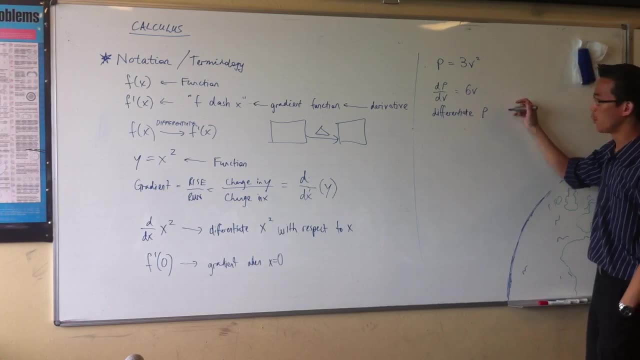 x is the um, the variable you're paying attention to Here. I'm differentiating p with respect to there's no, there's no x's in here. right, I'm differentiating with respect to a different letter, A different variable. 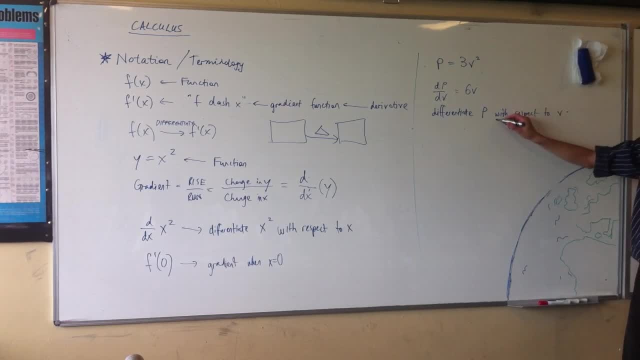 In this case, b- Okay. Sometimes you see that um, this abbreviated to this because people get sick of writing with respect to Okay. But there you go. I admit that's very confusing. There's so many different ways of writing it. 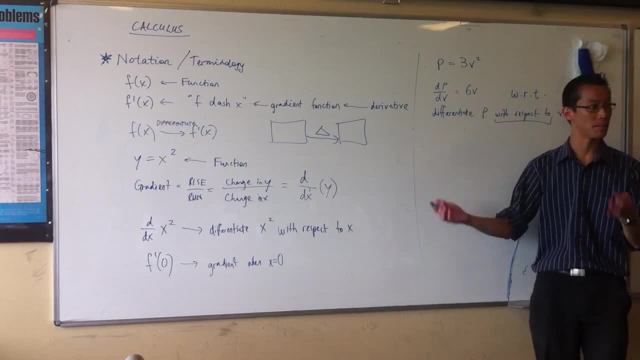 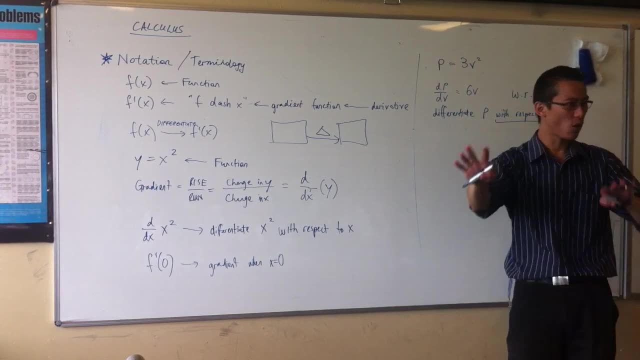 The reason why there's so many ways to write. it is because lots of different kinds of people- mathematicians, scientists, engineers, and so on and so on and so on- they all want to use this same idea, but in all their different fields they write things differently. Okay, So therefore you've got different notation that comes up because of it.